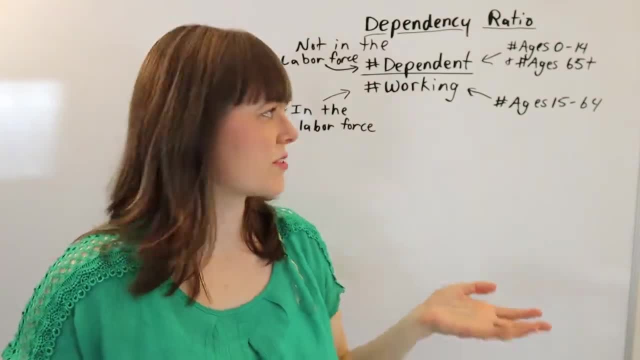 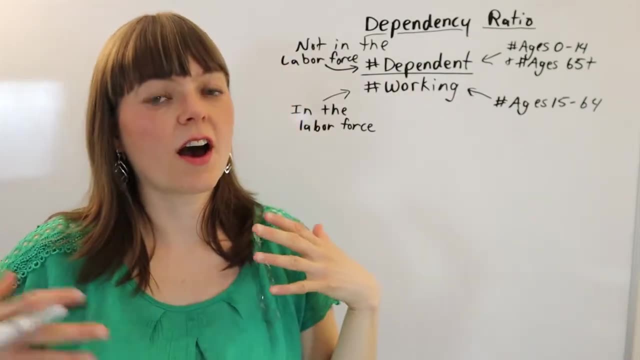 to account for people who can't work as adults, or people who are going to school, people who are raising children, people who are basically dependent on other people to support them financially, And to think this through more carefully. I think it's helpful to think back. 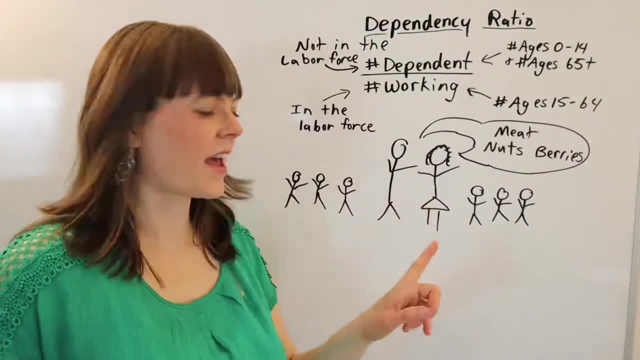 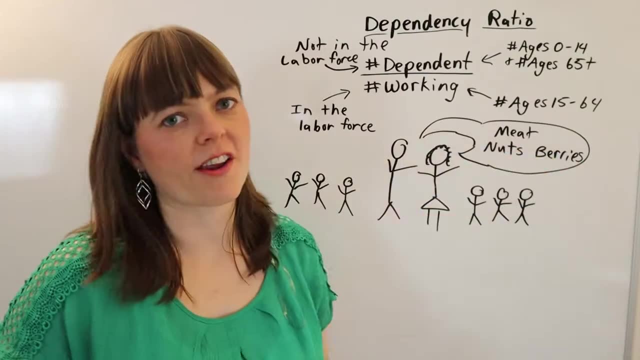 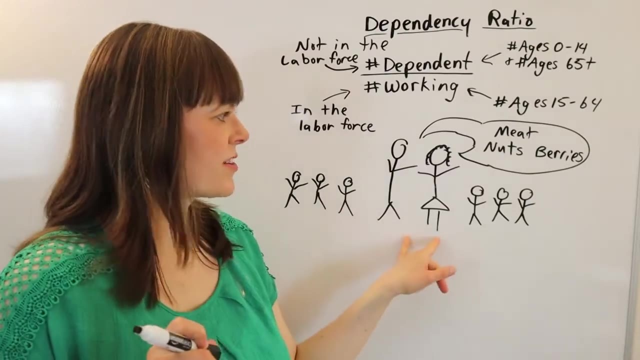 to the caveman era. So here we have a caveman and the caveman's wife and they have six children, And the children are not of an age where they can actually go hunting for berries or hunting for meat. So all six children are fully dependent, meaning the two adults are going to be out. 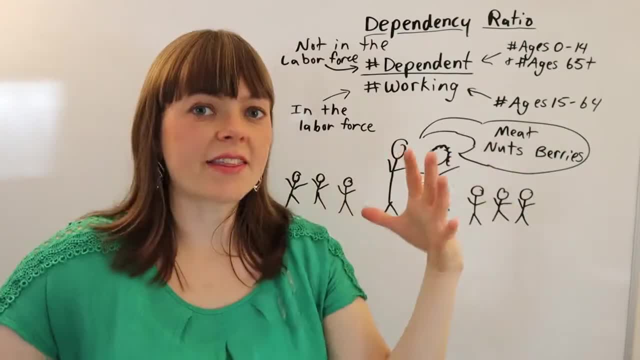 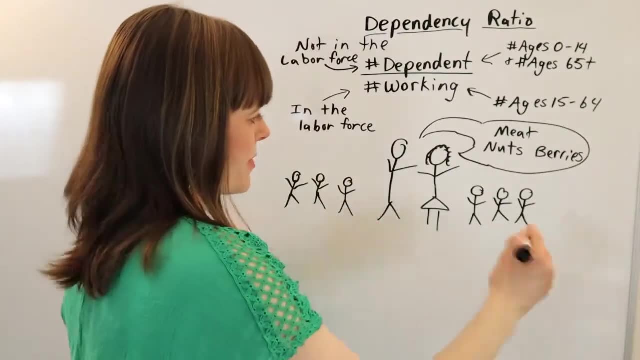 there collecting berries and nuts and hunting animals, And that pool of food and pool of resources has to be divided among the entire family. So in this case the number of dependents is six, The number of working adults creating the pool of stuff is two and the dependency 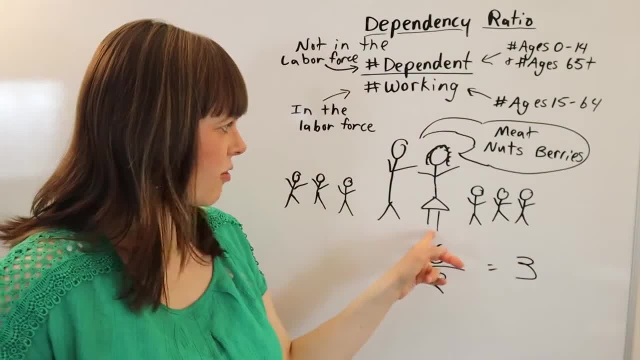 ratio is going to be six, And so the number of dependents is six and the number of working adults creating the pool of stuff is going to be three, Meaning each adult who's creating stuff has to be able to support three dependent people. 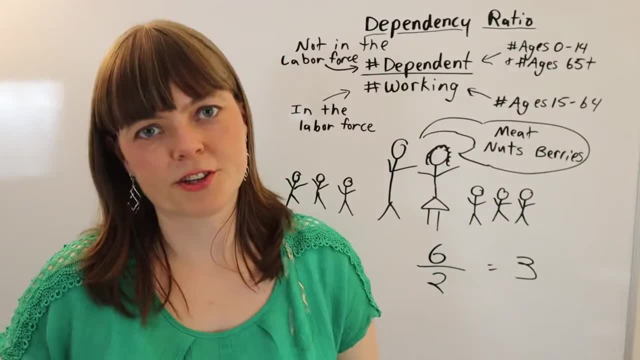 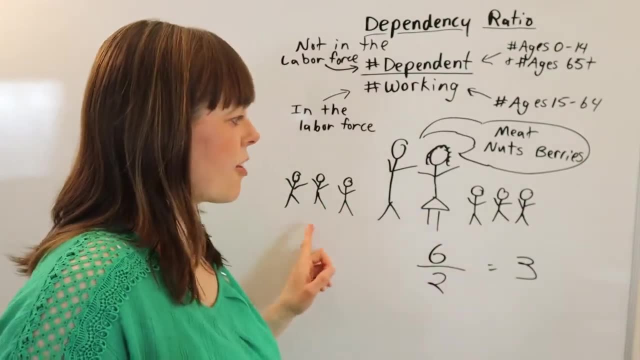 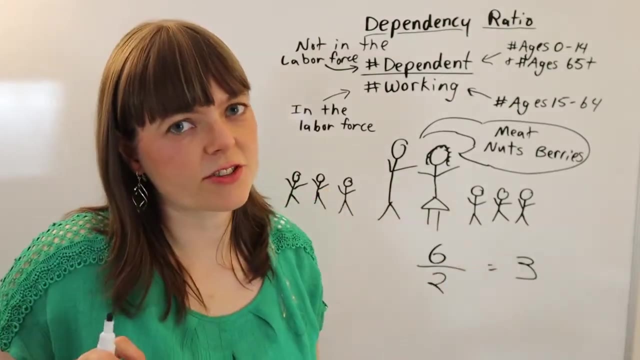 Okay, so that's the caveman version of the dependency ratio. Now, how does it differ today? Well, today there can be different styles of dependency. So caveman era, basically, the only types of dependents were mostly probably children And maybe occasionally an elderly. 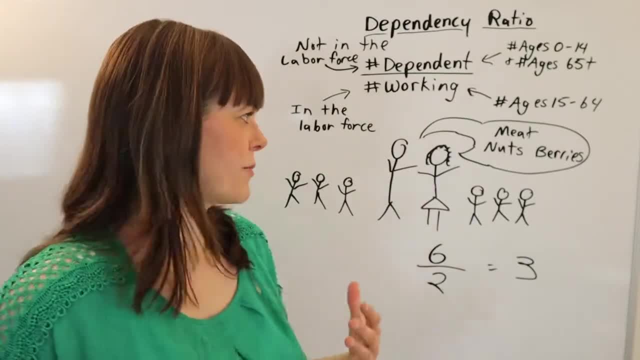 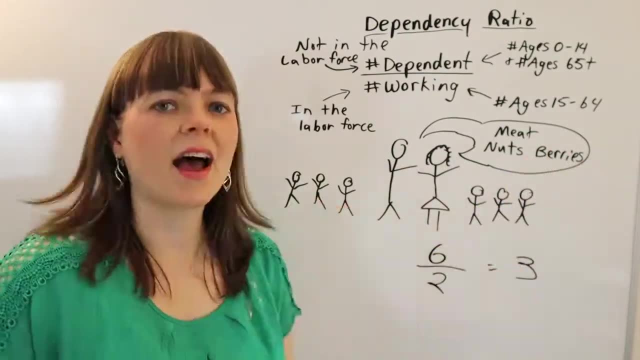 person who was perhaps wounded and could not care for themselves- So that's a different version of the dependency ratio- And could not care for themselves or could not contribute to the food supply, In which case that elderly person might also be considered as dependent in the caveman era, But most 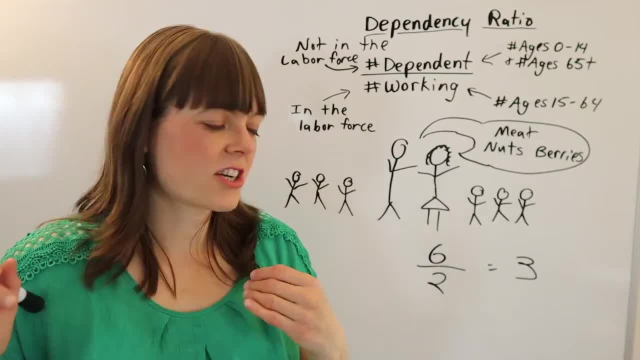 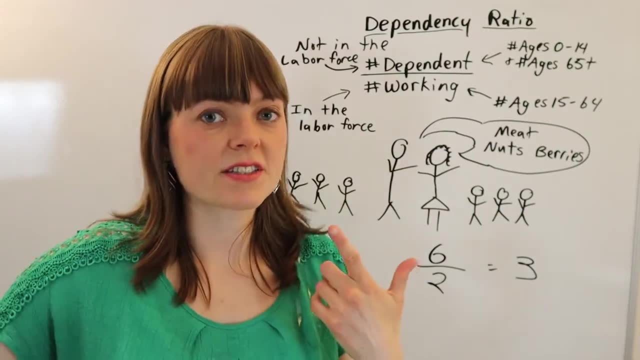 of the dependents at that time were children. Now we actually have different setups for dependents. One would be children, one would be older adults, for example a parent that you are caring for, And in both of those scenarios there's like direct caring for the person. 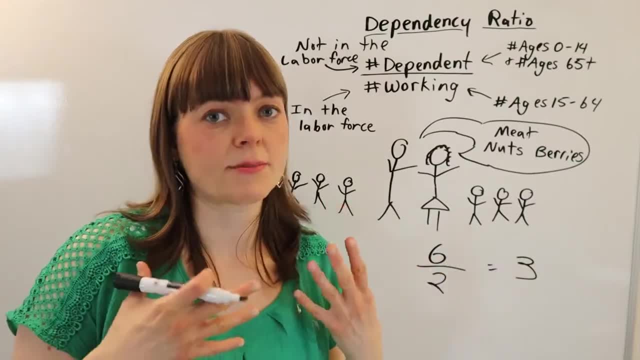 But there's also people in society who are more dependent than they are children, And so in my case it's not just children, It's also people in society who are dependent, perhaps on the government, perhaps on their communities, for survival, But they're not directly connected. 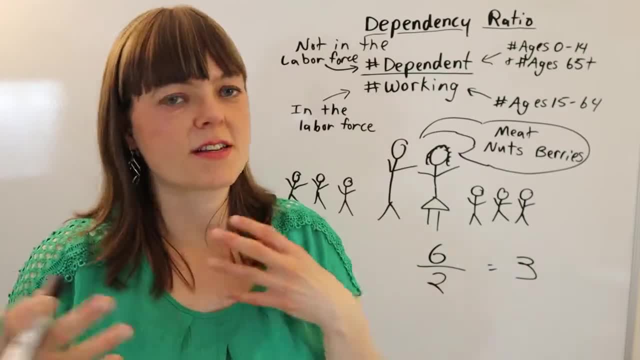 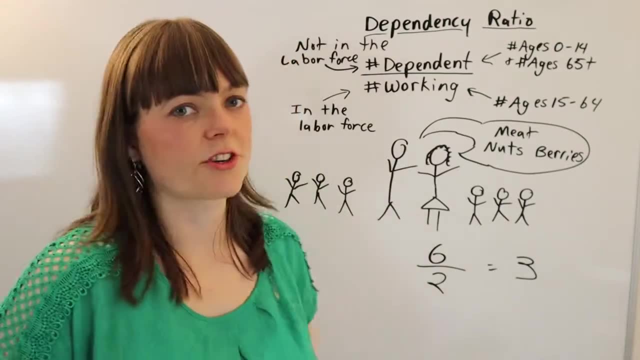 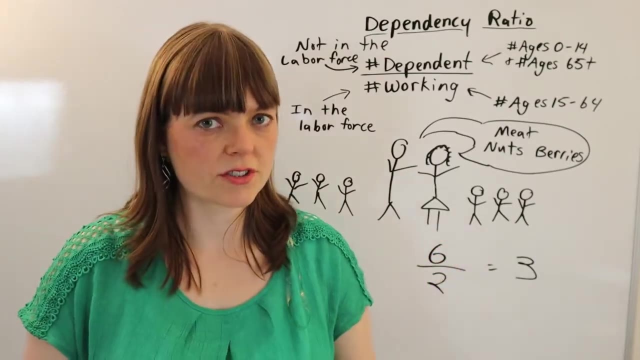 to particular workers, In which case the redistribution, the dependency is mediated through the government. And this is why economists think about the dependency ratio. We want to think about what is the burden of supporting other people on each working adult. Okay, and if you want to think about the dependency ratio in terms of the number of people who are dependent on each other or who are working in the community. that's not necessarily a dependent. It's just that we're using the dependency ratio to evaluate the burden of the job that we're putting in our lives and the side that's going to have to get increased. 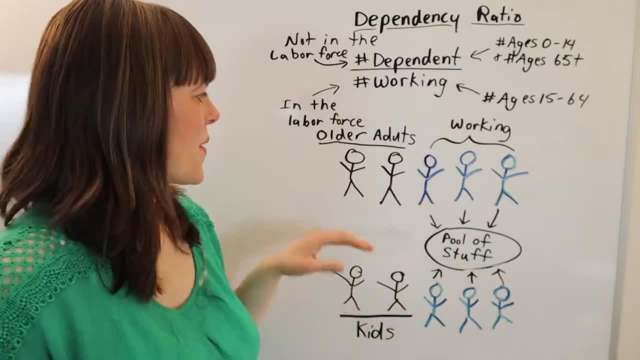 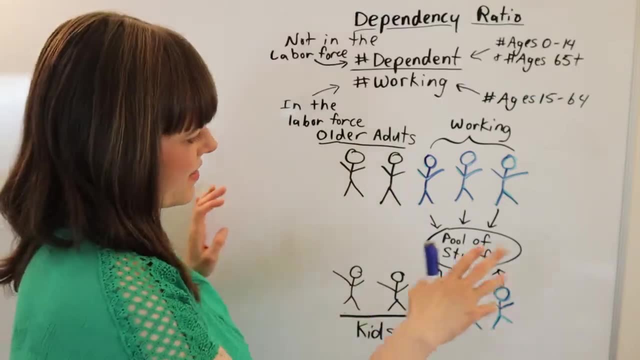 So that's a very important unit of information and we want to use it to evaluate the burden of terms of an entire population. we might have a 10% economy. that we're thinking about just to do a thought experiment And in this particular population I've set up, we have six working 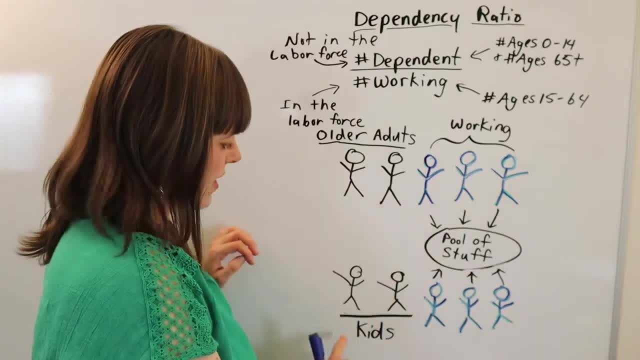 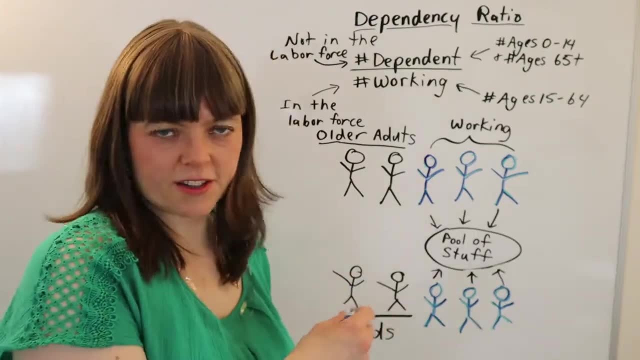 people, and two older adults and two kids. So these four are going to be the dependents And if you're going to calculate the dependency ratio for this particular economy, this is going to be four dependents, that's the older adults plus the kids. 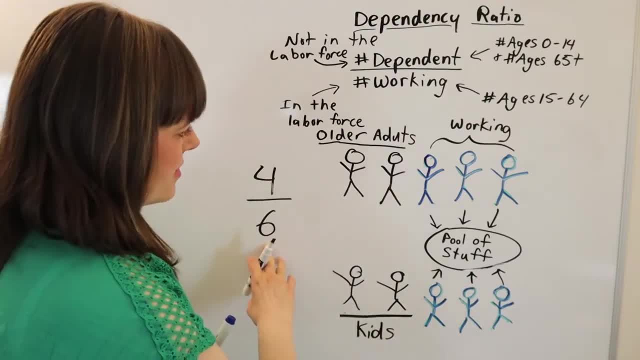 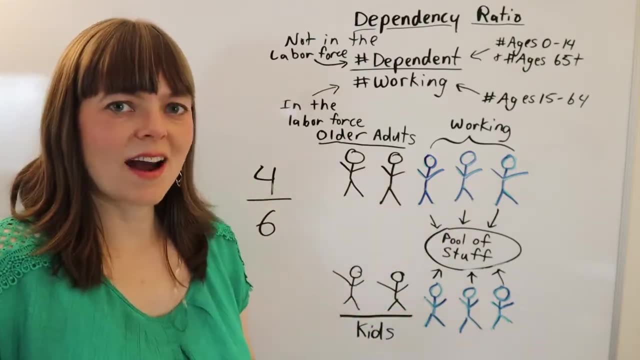 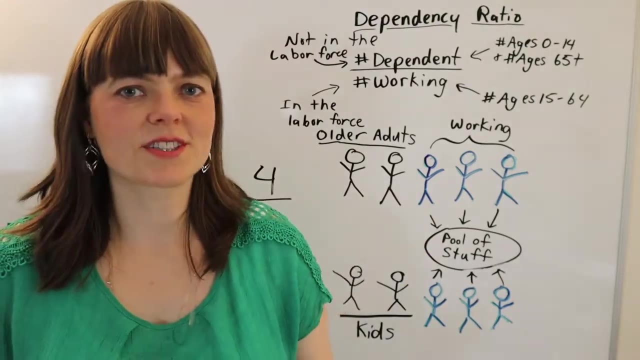 and that's divided by the six-person workforce population, In which case each working person has to support about two-thirds of another person. Now, one thing here is that we know that kids are actually a lot cheaper to support than older adults. Older adults are going to need medical. 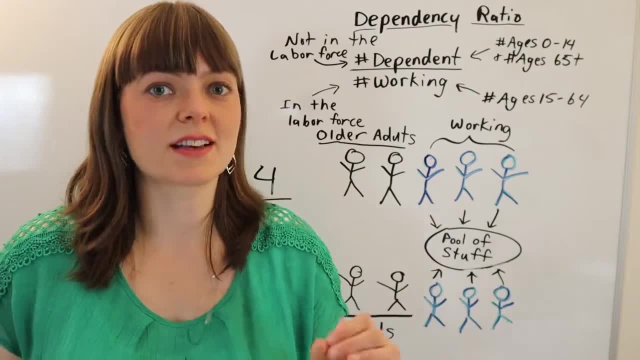 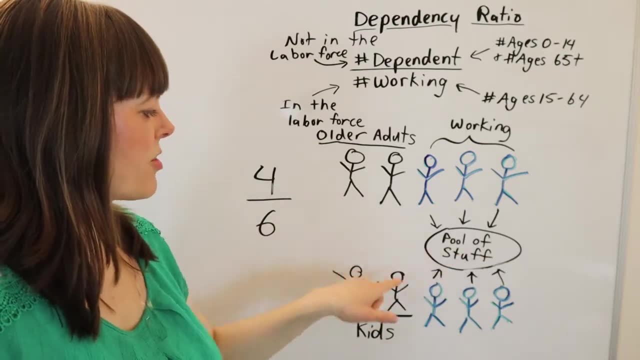 care they're going to need nursing home care. that's really expensive. Kids eat stuff, but they don't eat that much. So kids are going to be much cheaper to support on average per person than older adults. And that's divided by the six-person workforce population, In which case each working 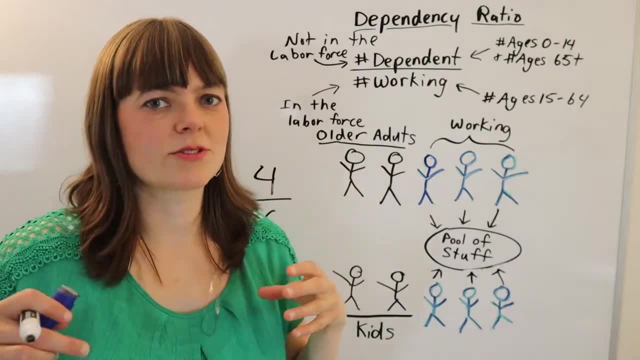 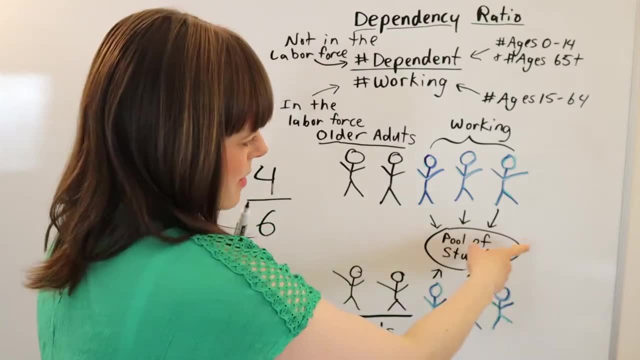 person has to support about two-thirds of another person, So kids are going to need medical care, which is why sometimes these dependency ratios get different adjustments for different types of scenarios like that. Now we imagine the pool of stuff that the six people are creating is going. 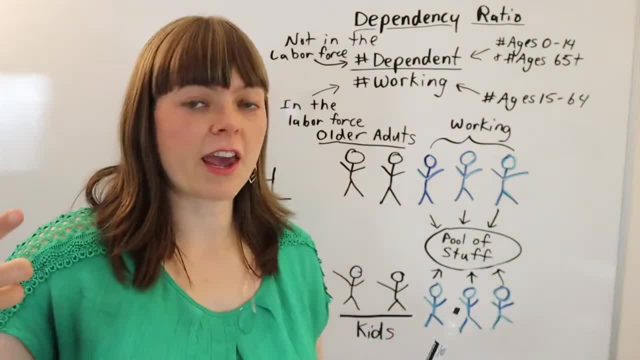 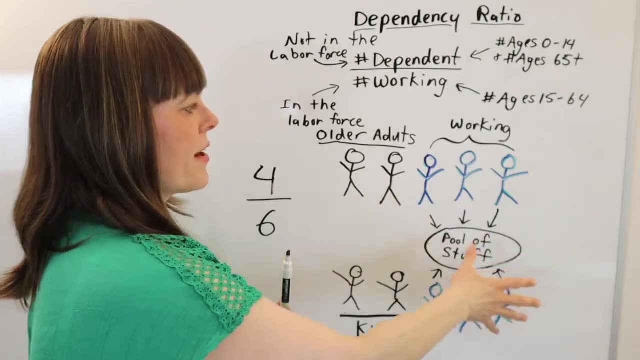 to involve food, it's going to involve healthcare, it's going to involve housing, it's going to involve entertainment. Everything that's created is what gets distributed among the ten-person population. So if we imagine a situation where the six-person workforce population is going to be, 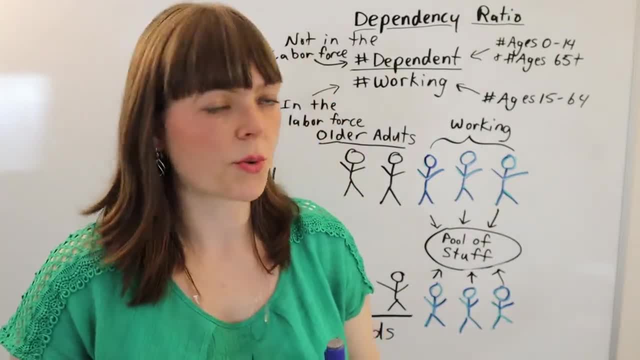 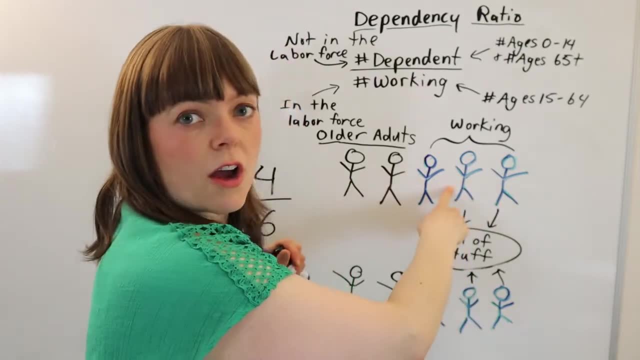 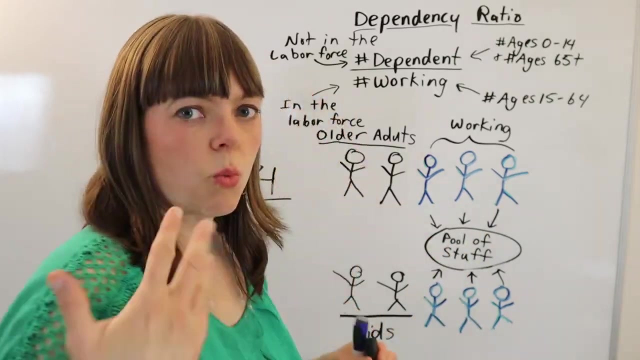 divided into two parts. we have an aging population, as many countries do, and the dependency ratio is going to go up. For example, let's imagine that these two people are about to enter into the older adult community. they're about to quit the workforce and retire. In which case, what happens? 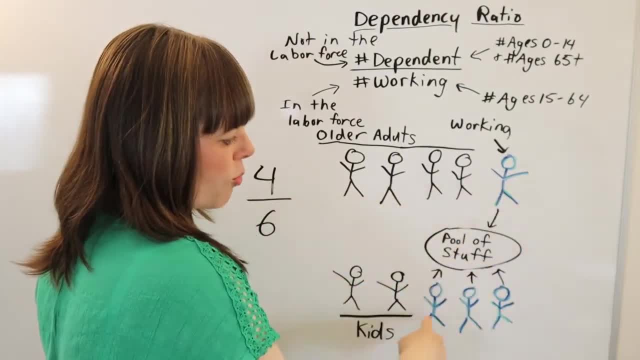 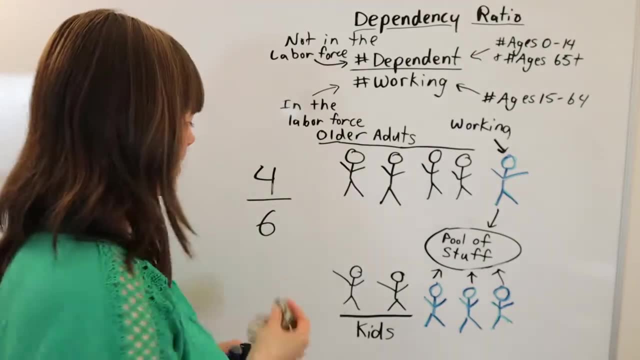 Now, suddenly, we have four older adults, we have four working adults and two kids. So let's recalculate the dependency ratio and think through what this means. So six dependents now four working people. Previously, each working person was supporting: 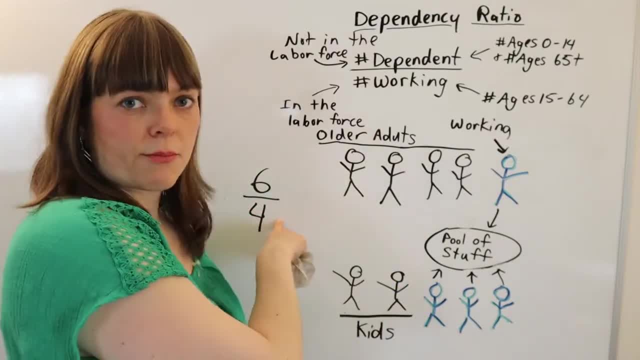 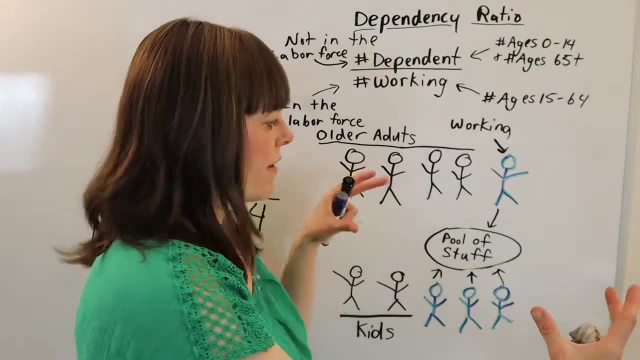 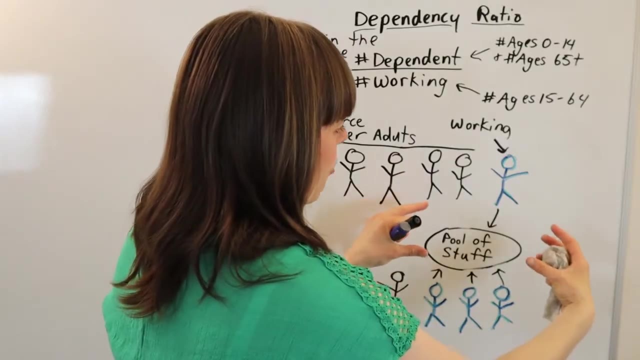 about two-thirds of another person. Now each working person is supporting about 1.5 other people. The other thing that happened here is that the pool of stuff got smaller. We used to have six people working to produce food and housing and clothing, and now we only have four. 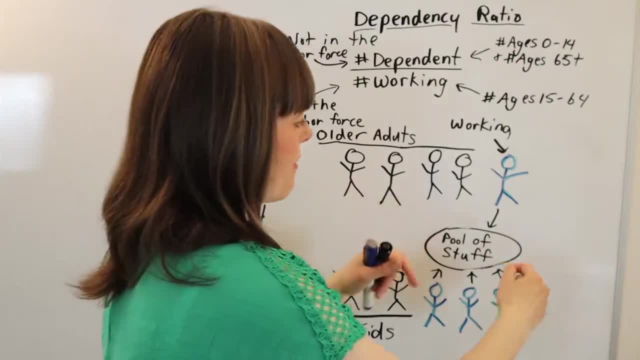 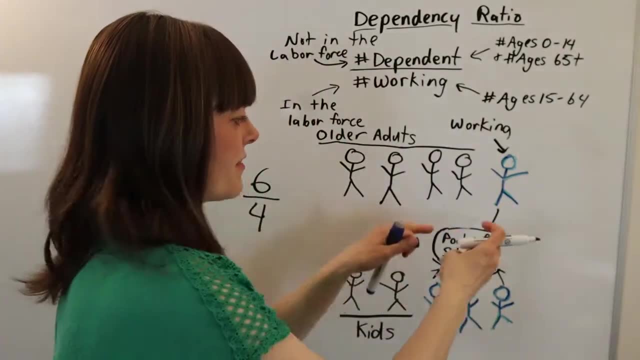 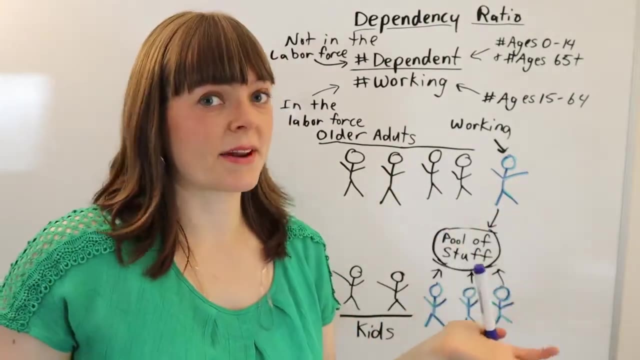 So because what matters is not money but actual stuff. we know that the pool of stuff to the support the population just got smaller And yet that pool of stuff still has to be distributed among the 10 people in that society. And this is why the dependency ratio matters, is because we want to know what's the ratio of the 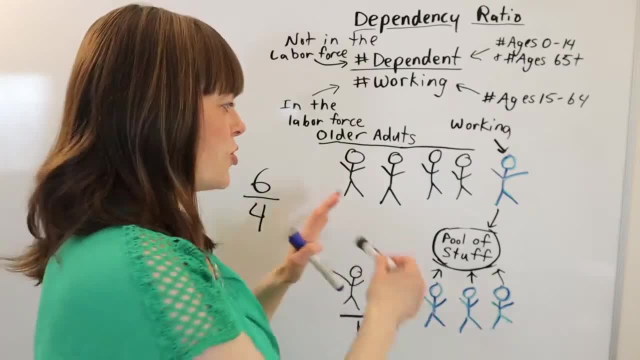 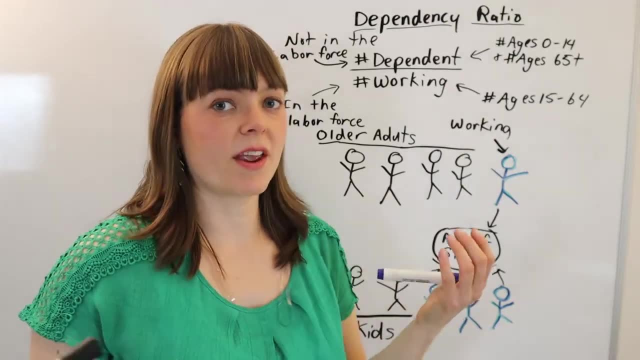 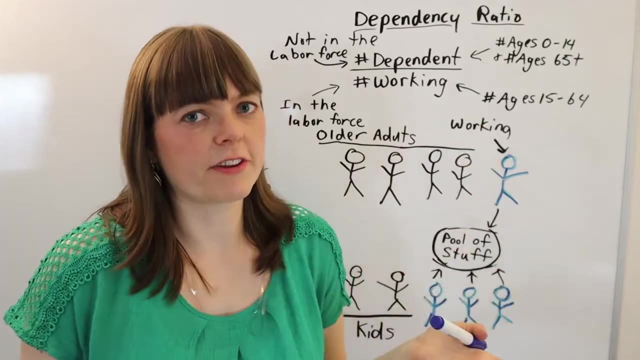 pool of stuff that we create in our economy to the people who need that stuff. And one thing about stuff is that some of it can be created and then stored up. For example, you can build a house today that's not going to be in use for another 50 years. that might not happen. 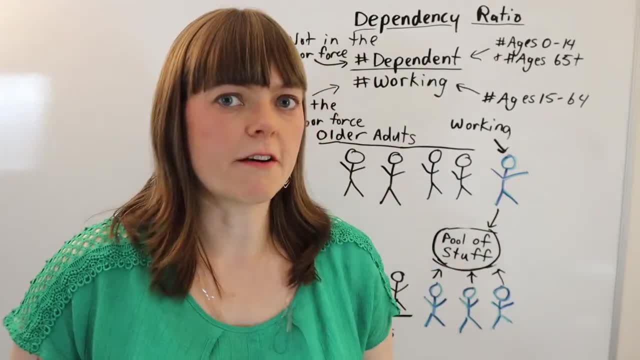 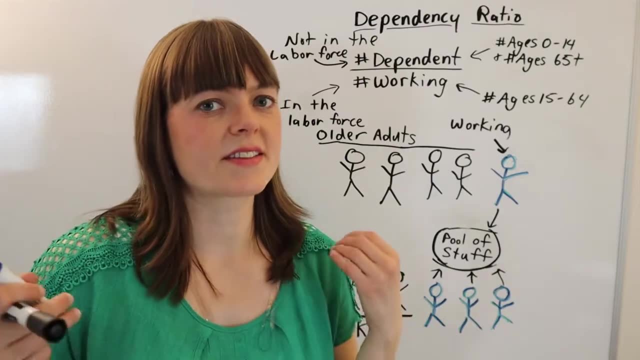 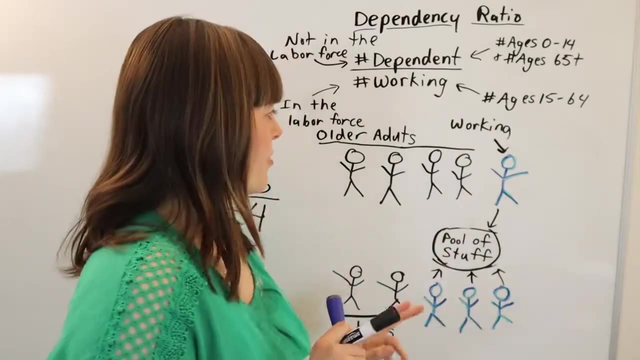 very often, but it's at least possible. well, other stuff like food and medical care and services of all types pretty much have to be consumed in the same period when they're created. so you can imagine one thing that you can think about through the dependency ratio is inflation. let's imagine these two people. 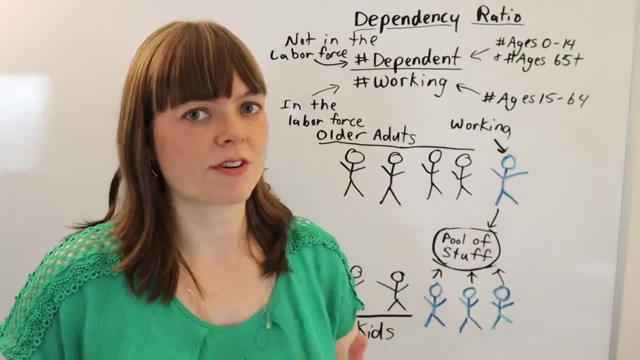 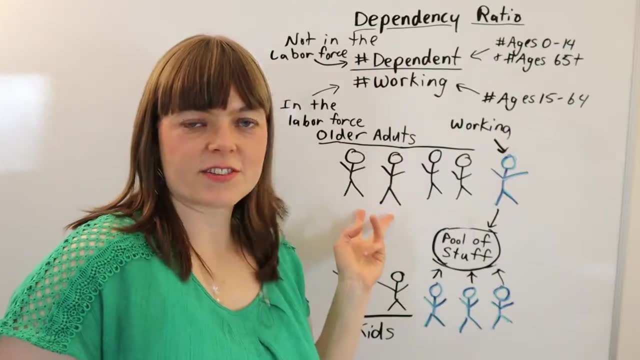 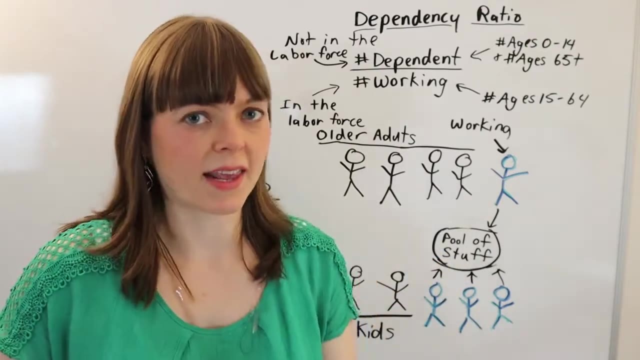 who were in the workforce population. they're saving up for retirement. they're trying to figure out how well off will I be during retirement and to do that they're looking at these older people who had saved up money over their lifespan and they see how much stuff these people can buy with their money. the problem is if these people save up the same amount and then retire and the pool of stuff in the economy shrinks because we have more people in the elderly population, what happens is that the people who are in the workforce is the same amount of money can buy less because the money is sort of evenly. distributed across the population, at least in our thought experiment- but the pool of stuff got smaller, so it's more expensive to buy any one given thing, which is why the dependency ratio is one thing to think about if you're thinking about inflation and if you're thinking about population level changes and how. 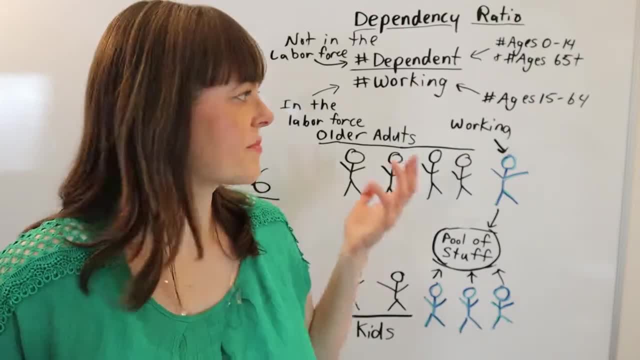 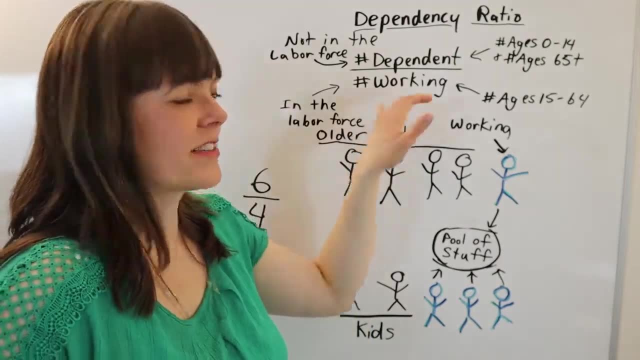 that's going to influence the economy. all right, you're going to have to think about how you're going to influence the economy. so I think that's a basic overview. I think that's all I'll say for this video, but the basic idea here is: there's many, many ways of constructing dependency.